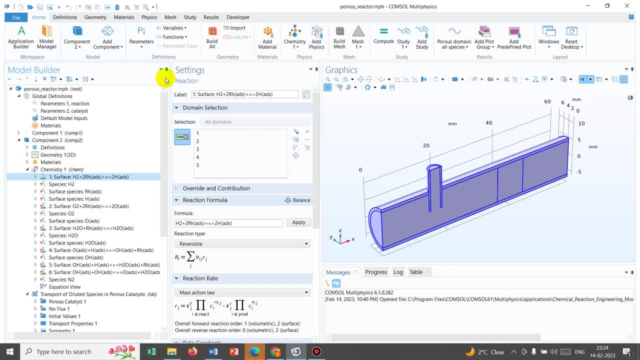 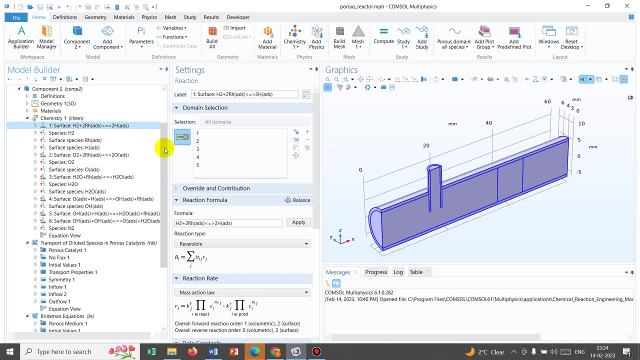 the special kind of reactors like plug flow reactor or mixed flow reactor, CSTR or whatever. So in this kind of reactor, which is porous reactor, what are the physics necessary? So initially they have taken chemistry. So you can understand why chemistry is important. because in a reactor 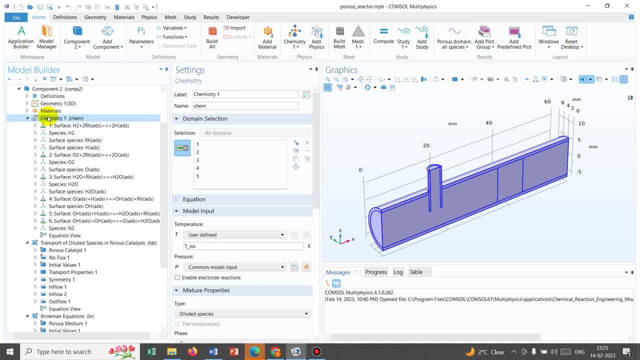 there might be multiple chemical reactions going on at a time, So you actually have the provision of enlisting all the chemical reactions under the chemical chemistry option. This is the physical reaction. The name of the physics is chemistry. So here you can see. they have noted down all the 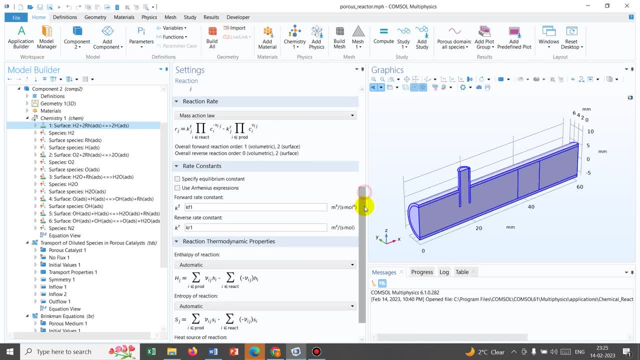 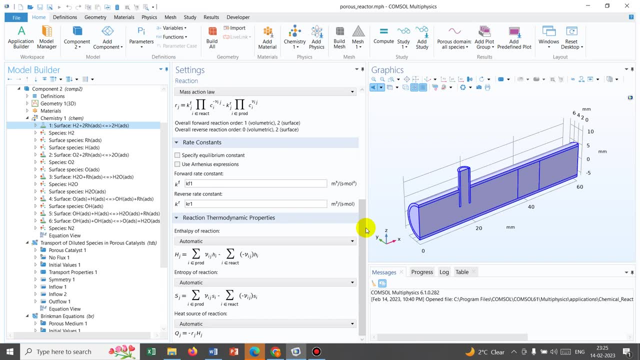 reactions and the parameters. that means the rate constants and other parameters. If it's a reversible reaction, then it has forward rate constant. it has backward rate constant. Like the way you can see, this is a reversible reaction. So they have defined Kf, that is, the forward rate. 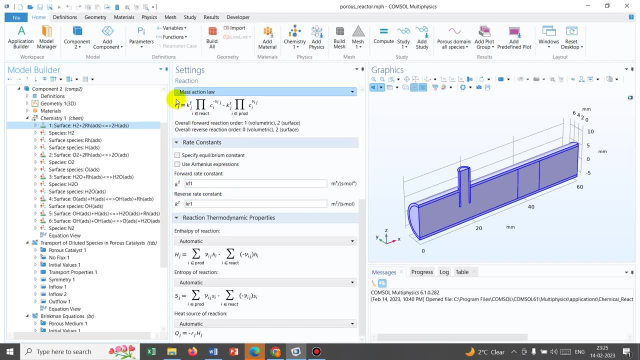 constant. the backward rate constant. Overall rate of the reaction is defined as this. You can see this is Kf forward reaction rate constant. This is the multiplication symbol. that means if you have n number of components, say C1, C2, C3.. So multiplication of C1 into C2, into C3,. 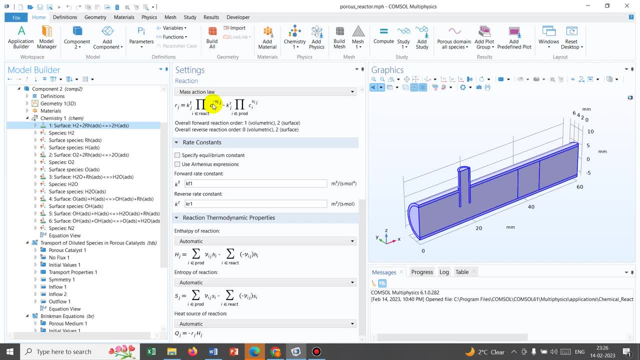 and we actually know these things are experimental matter. that means chemical reaction, kinetics. it comes from the experimental observation. So if you know about the reaction then you can know about the reaction rate rate, constant and everything, and from those known parameters you have to define it under the chemistry option. So 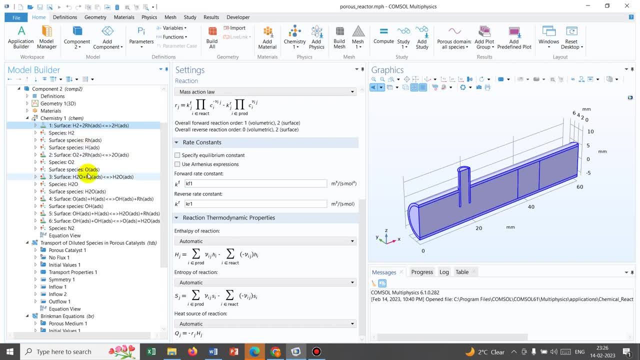 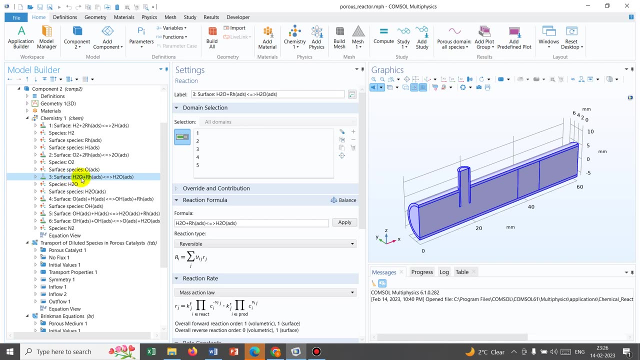 this is a reactor wherein the hydrogen evolution and the reaction between hydrogen and oxygen goes like even if you see here, So on this particular surface, what's happening, this is H2O on rhodium surface. It is giving you adsorbed H2O. that means you have a catalyst. 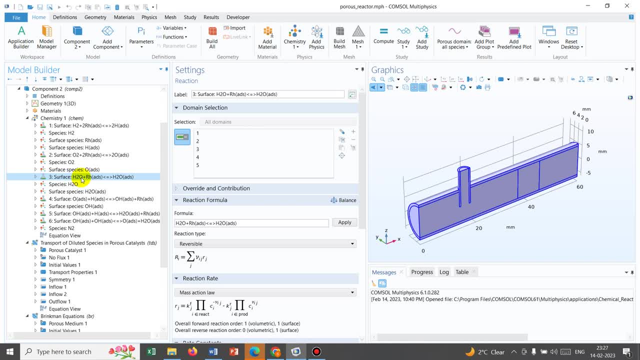 and if you put water on top of that, then the water molecules may be embedded on that catalytic surface. So if this particular process also has some reaction rate kinetics, so they have taken for this. If we look into some other reaction like this one, 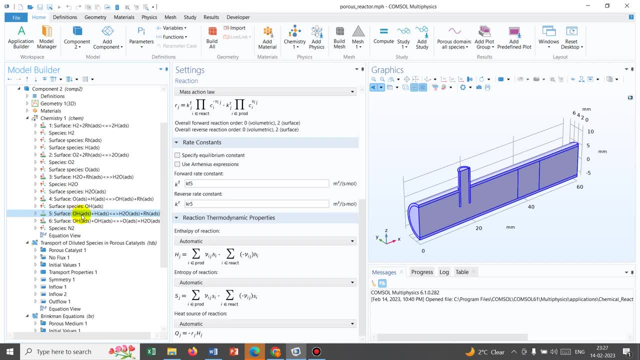 you can see this is a reaction between OH- maybe it's a radical- and the H radical which is giving rise to H2O on the rhodium catalytic surface. So you can see when, inside a reactor, there might be multiple steps happening and if you know about those steps clearly. 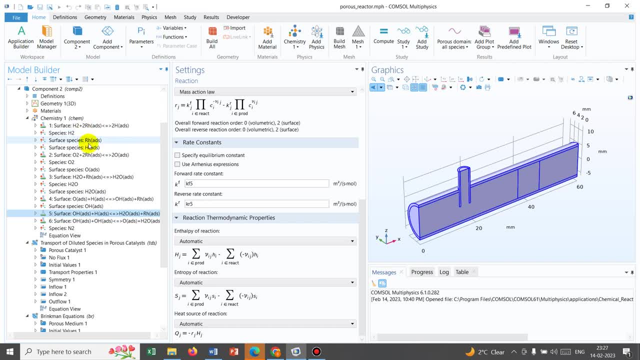 then you have the option to unleash those properties. So our target is not to understand this particular chemical reaction which is given in the puras reactor of Comsoll MultiPhysics, but to understand which are the ways by which we can define a chemical reaction. 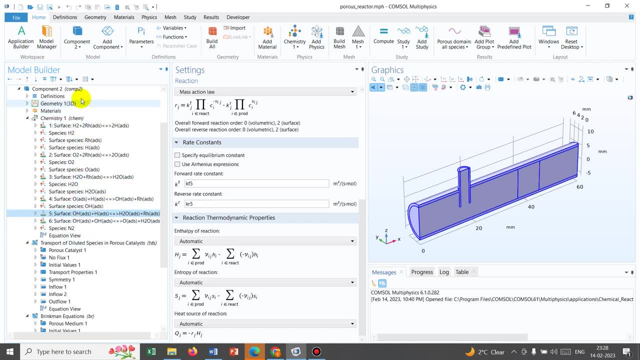 or a chemical reactor. So this particular physics, which is chemistry, is taking care of the several reactions, and that's several of those reactions. so between H2O, of carbon dioxide, which generally does not release or actually reviews R socket, or the reaction which need a melamine- blah-bl работать. 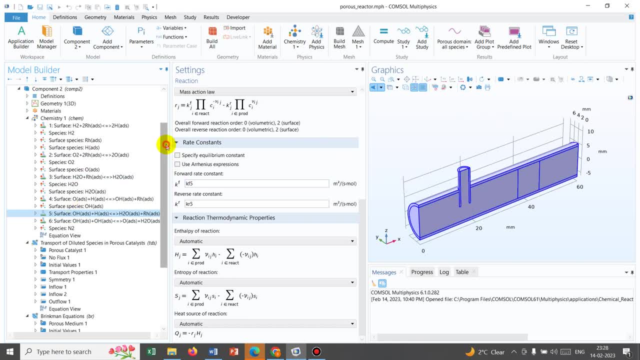 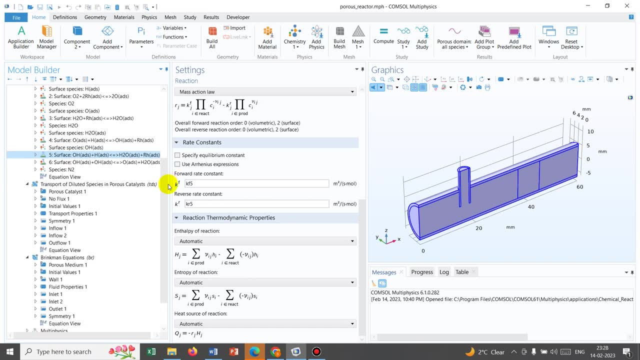 with a detection of sulfur, or rather, according to that, that is very high Bieber chemistry at which kiemREAM or that goes on inside the reactor. so once we define it, then we go for. so what's happening? this is not only the chemical reaction that takes place inside a reactor. there might be a flow coming in there. 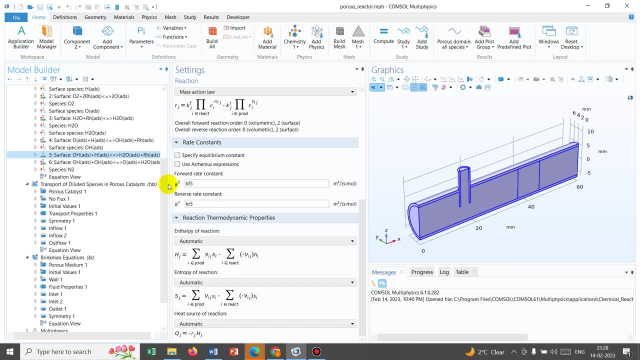 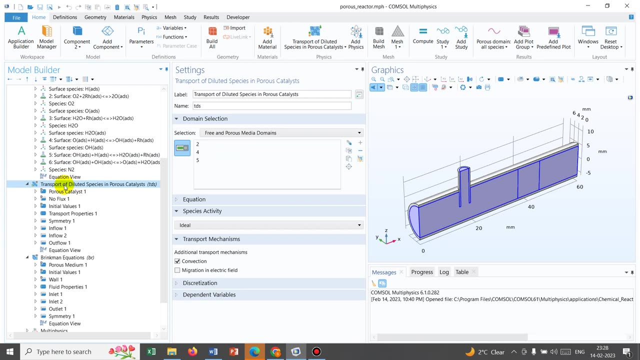 might be a flow going out, so an inflow and outflow in the middle reaction is happening. so this inflow and outflow, that physics also we need to take care of and that comes from this TDS, that is, transport of diluted species in porous catalyst media. so this physics is available in Comsol, as this is a 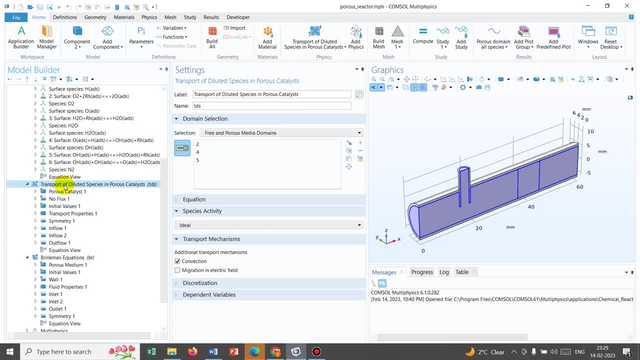 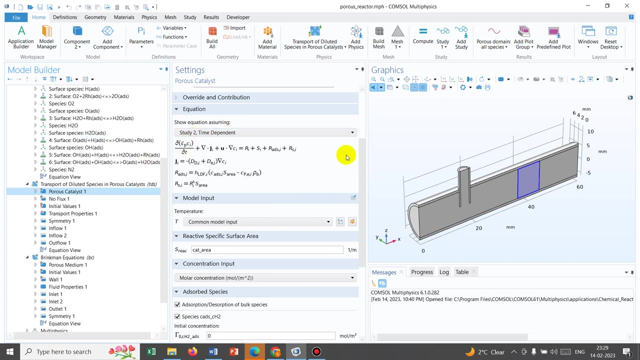 I mean, this is a, this is a reactor and a porous catalytic reaction is taking place. so in Comsol there is an inbuilt option of porous catalyst, so they have taken this particular option. but today I will show you how to do this. I am not going into the details of the equations, because in all of my videos I emphasis on 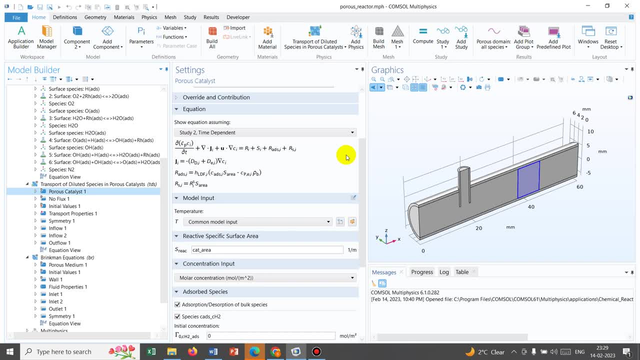 chemical on the equations, but today we don't have enough time to discuss about each and every equation because there are multiple equations enlisted. but I'm just trying to initiate the discussion and from the upcoming videos will be taking several cases and will do different case studies so that it becomes very easy to comprehend. So they 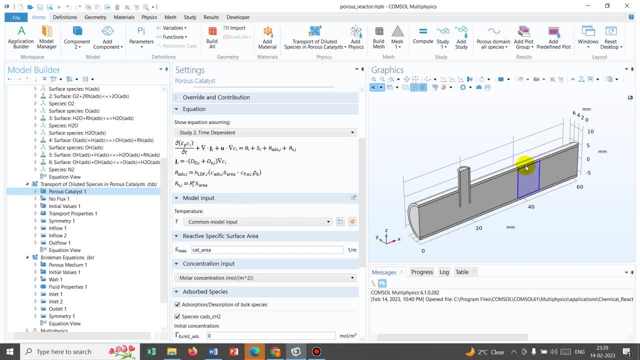 have taken porous catalyst. so this is the part I mean. in a reactor there might be a particular zone where the porous catalyst is kept, so you have to define this particular zone. if you see, they have actually defined the catalytic portion. Now they have defined inflow, outflow. there might be multiple inflows. 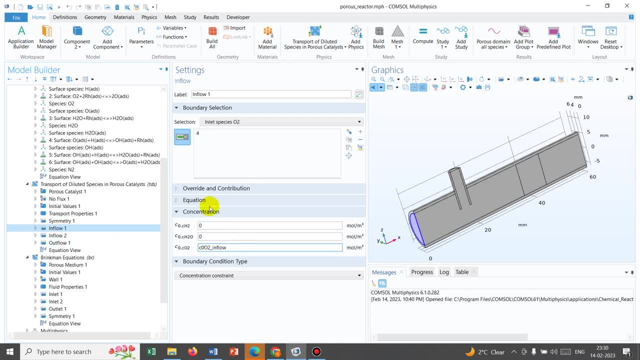 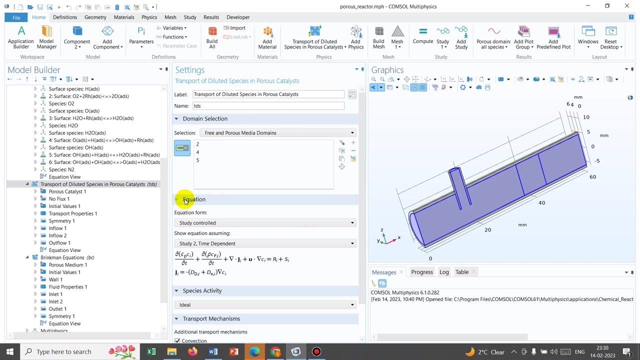 like this case, they have two inflow and the conditions of the inflow may be different. you can see from those boundary conditions, inflow is different from the inflow to and at the outflow. this is the outflow option now this transport of diluted species. it takes care of the concentration throughout the 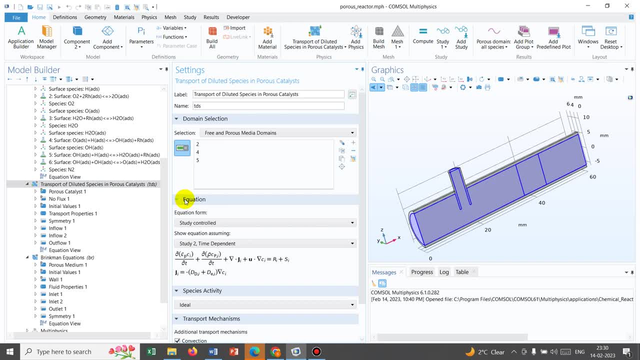 reactor. there might be multiple components, so this particular physics takes care of the concentration throughout the reactor. There might be multiple components, so this particular physics takes care of the concentration of multiple components inside the reactor. but there is a flow associated with it. but this flow is not very similar to normal laminar kind of flow, because the flow 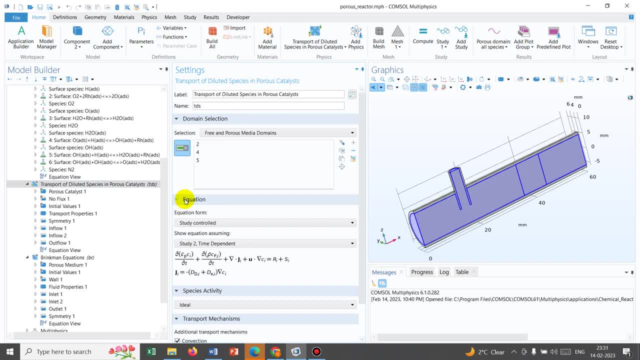 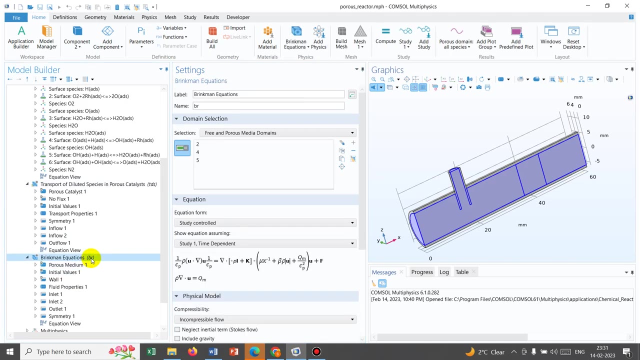 is happening through the, through the porous media. so for that, in order to model porous media flow, we need an appropriate physics. and for this case they have taken brickman equation. so i'm just discussing, i'm just telling the name of the equation today, i'm not going into the details. 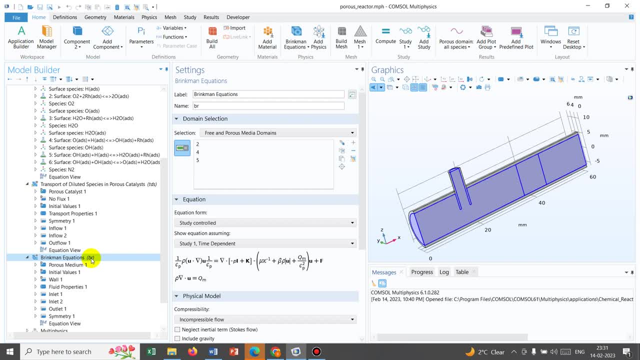 of the brickman equation. but we'll study on it. we i'm studying those equations, so in the upcoming videos i'll come with this physics so that many people tell me to model porous media flow. so i started working on it. i'll be understand. i'll try to understand the physics in detail and then in the upcoming series,